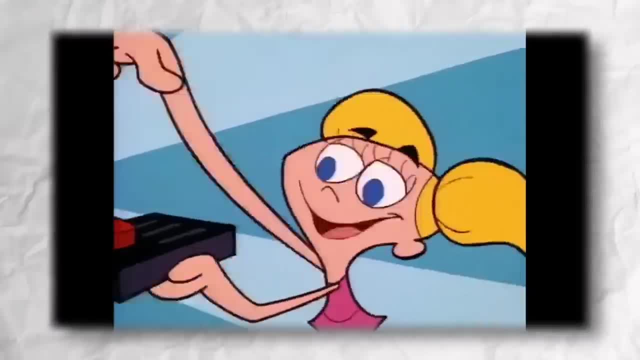 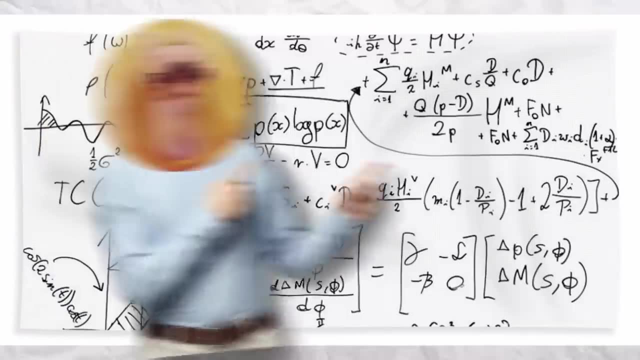 animation. Is AI going to take our jobs as animators, And can you actually get animation with one click? Well, I recently found a new software and put it to the test to see what it's really capable of, And let me tell you, the results at the end of this video are pretty. 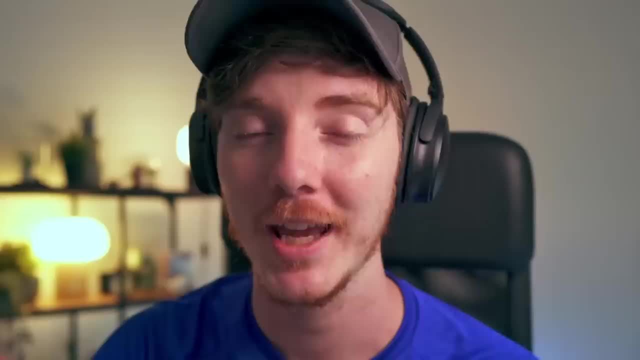 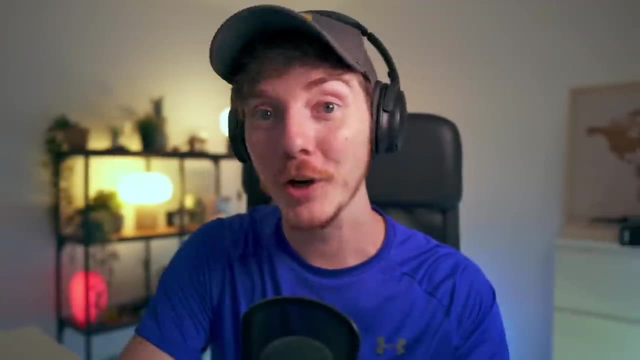 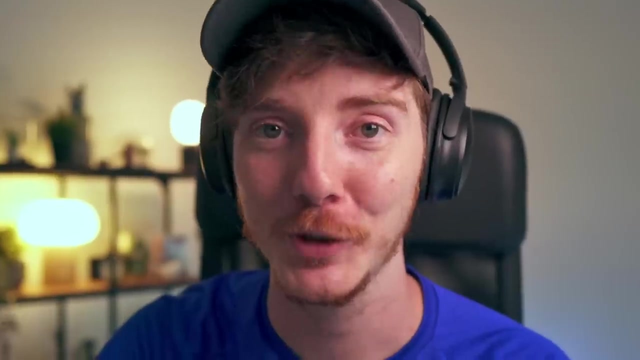 insane. So I want to break down some of its best features and hopefully show you that it's not all doom and gloom. The software I'm talking about is Ascadar, and it's not often that you get to see a whole new animation software come around. I mean, look at this. 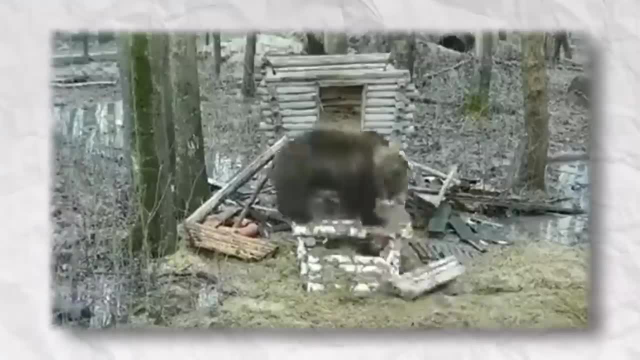 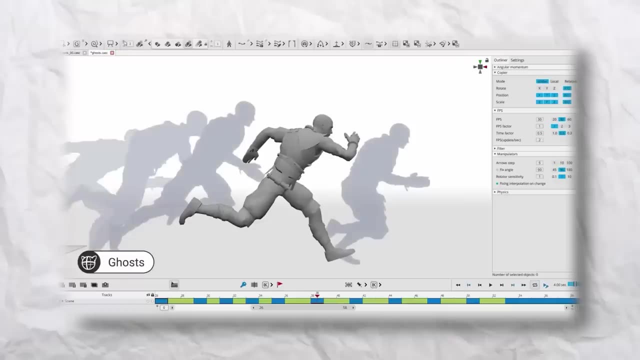 So, basically, a small game company named Neki has developed and released this software about four years ago. However, only recently was this software released to the public for free. Every single aspect of this thing is free for you and me to abuse. Essentially, 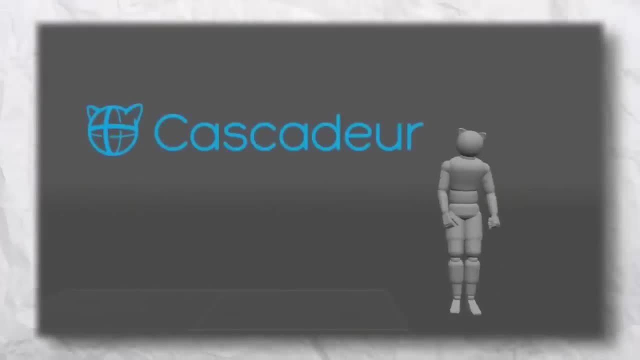 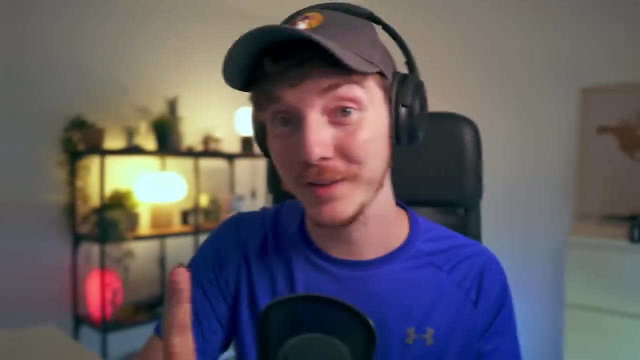 it's an all in one animation suite and has everything an animator might need, from the graph editor all the way to rigging. This thing is a super powerful tool, But the main reason why this came onto my radar is because of the AI assisted features. 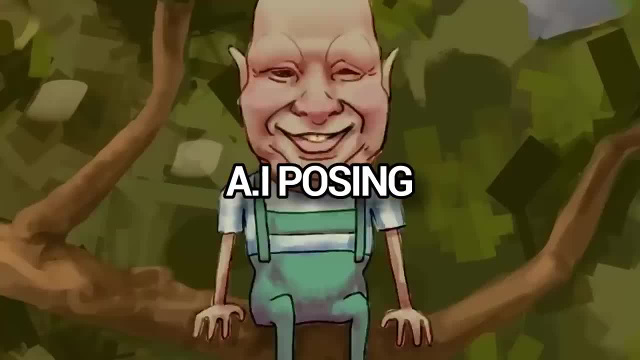 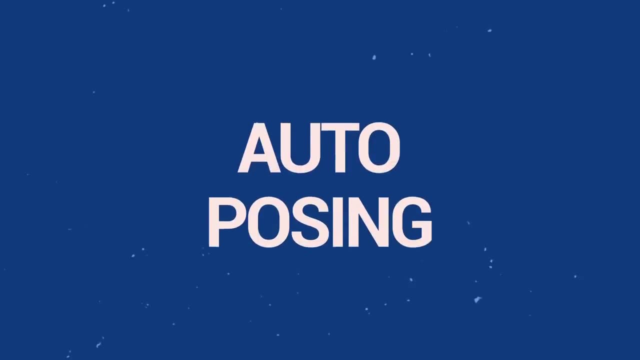 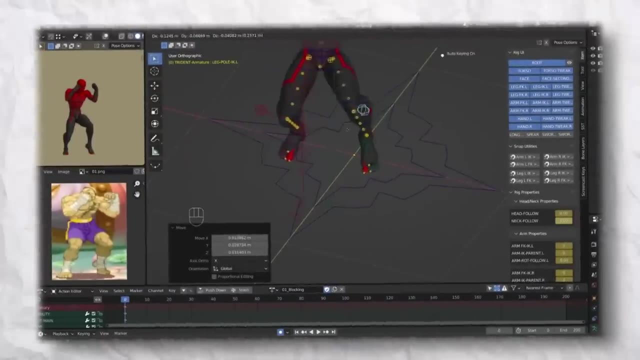 So let's cover them quickly. I'm starting off with the heavy hitter: auto posing. When I first started playing with this feature, I thought it was just some kind of gimmick, but it's actually super powerful. So generally, when you're creating your key poses, you jump in and set up your character. 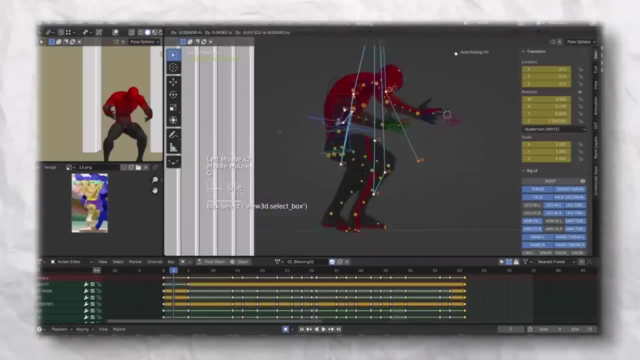 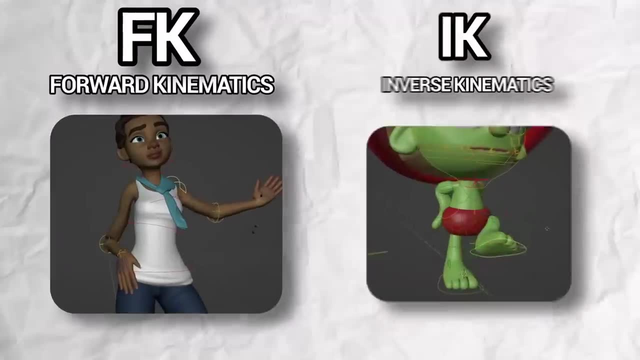 joint by joint in the position you want. You then set up a keyframe for each major pose and then move on to the other stages, like splining and polish. Usually there'd be some FK or IK controllers that you can switch on and off. 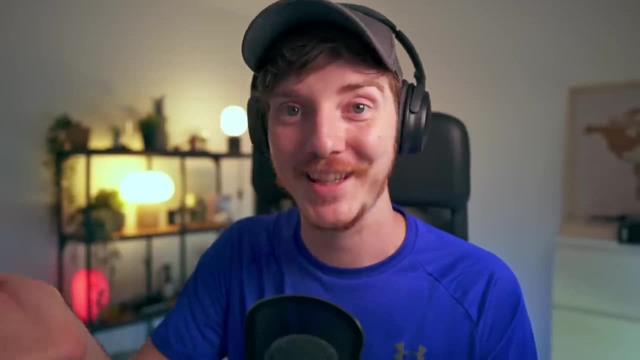 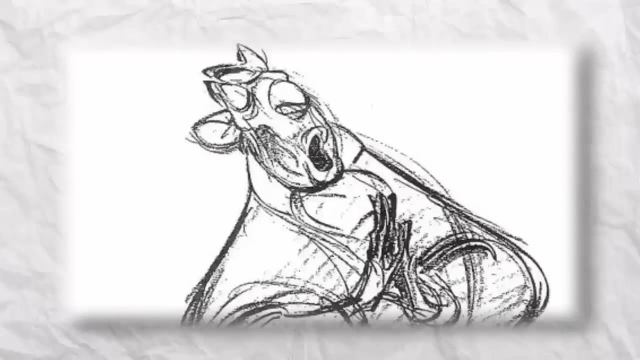 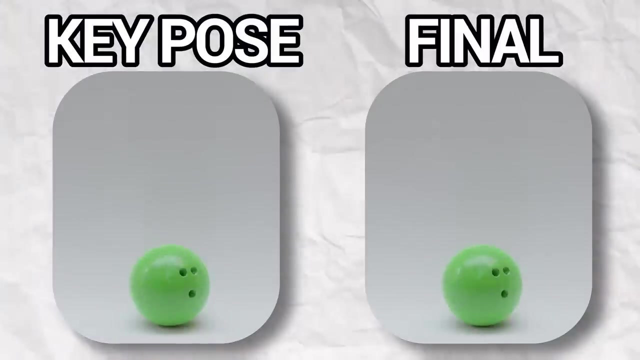 but, generally speaking, this is the process. As you can see, it takes a while and, honestly, getting the key poses down is extremely important, as these determine the major actions of the shot. It basically shows you, in the most minimal information possible, what the actions and movement of the animation will be. So with Cascader, 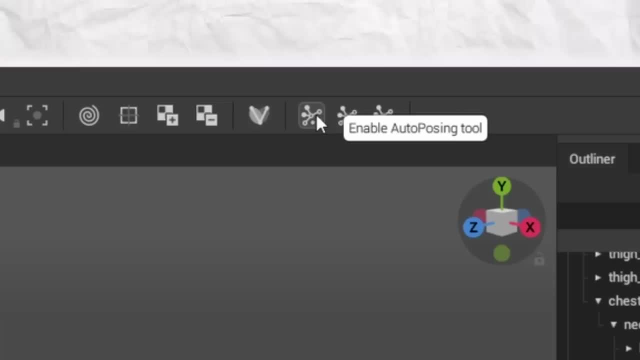 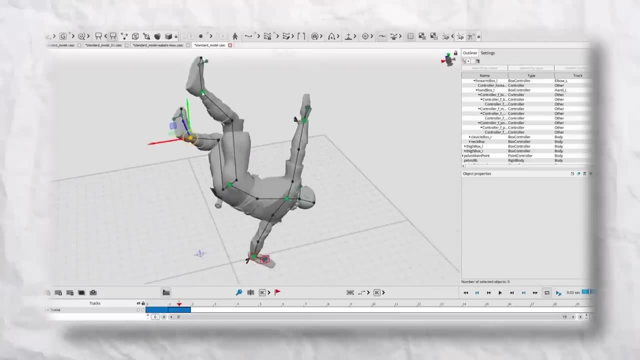 they actually have a setting that you can toggle on here, which is called auto posing. This is where you can set up your key pose and then move on to the next key pose. So, for example, I can move the legs or the arms and the whole rig follows suit. 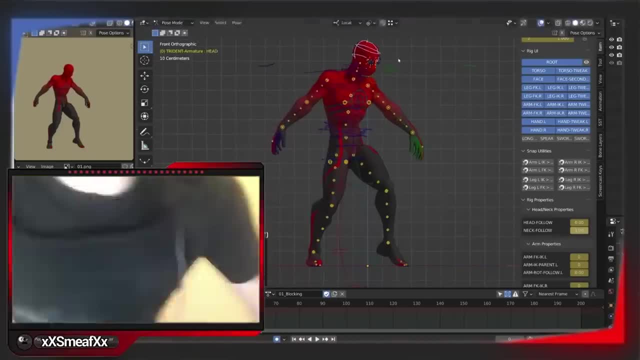 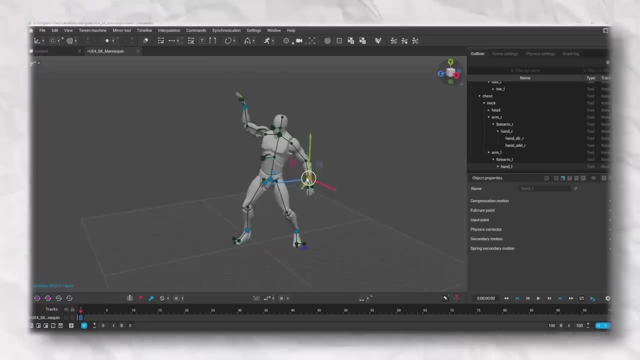 Instead of painstakingly moving each individual joint, I can simply hit this button and automatically the best physically accurate pose gets created in seconds, which is super powerful. So with this tool enabled, I'm able to set up a super simple block out of my animation. 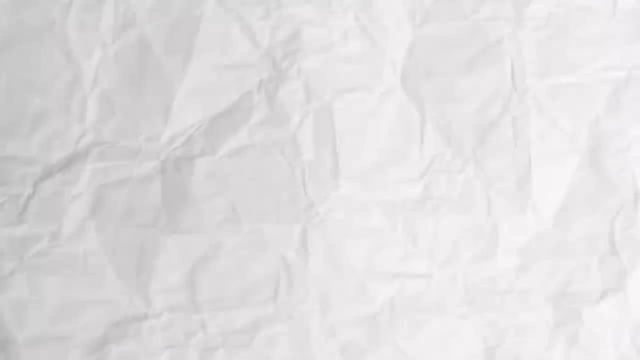 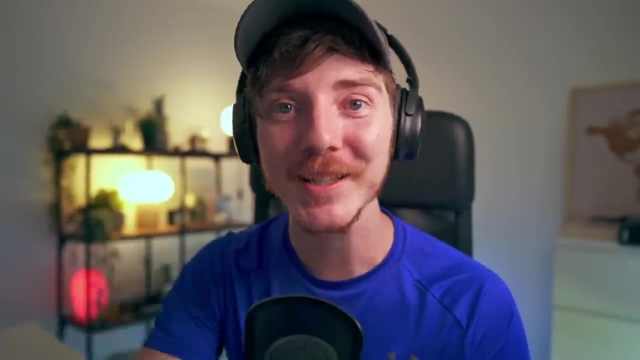 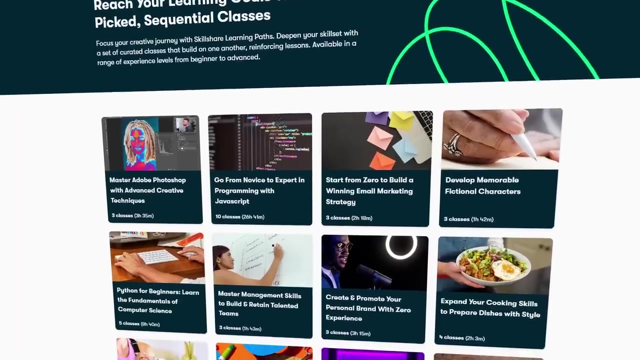 and it's way faster than the traditional workflow. And speaking of time savers, I want to show you my favorite platform to learn new skills And, yes, this is sponsored by Skillshare, but I want you to stick with me here, because I think you're going to get a ton of value from this. Skillshare is an online learning. 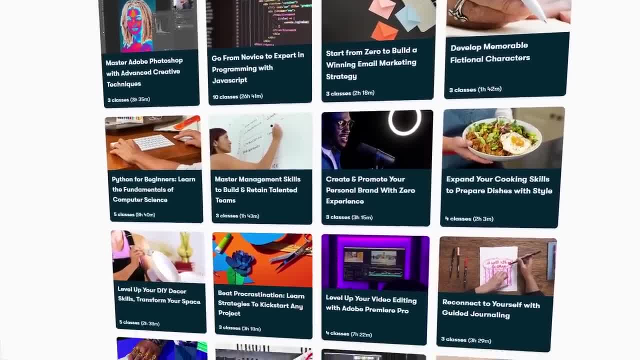 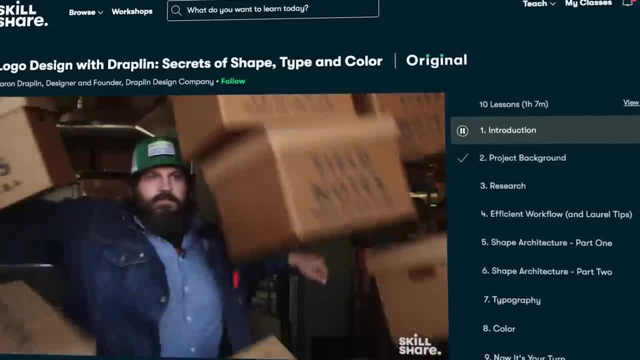 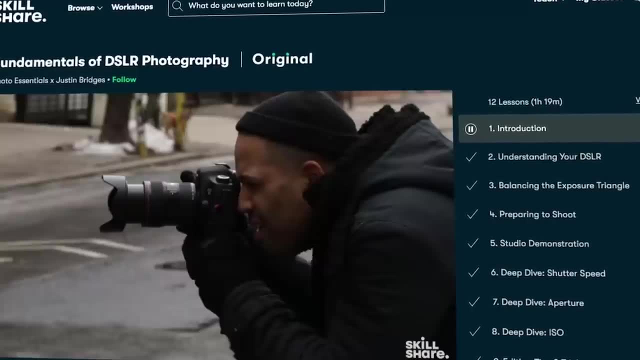 platform curated to show the best of the best creators, whether it's 3D, logo design or even cooking. they have literally thousands of classes to offer. Not only that, but it's entirely ad free, and it's a great value once you start digging into the classes that are actually available on here. 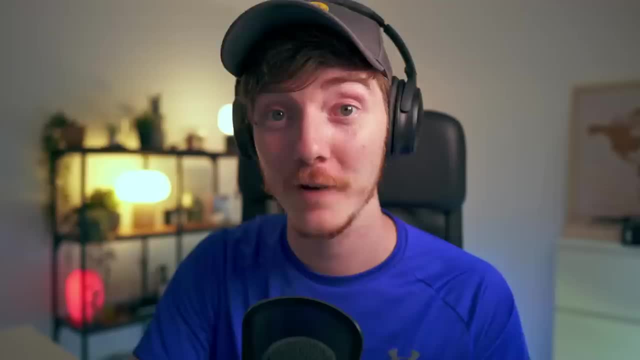 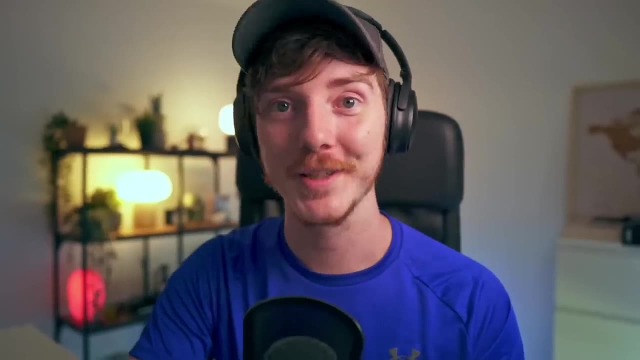 If you're watching my videos, you probably already know half the creators here. For example, there's Southern Shoddy, Bad Normals and, hey, even this guy- he seems pretty cool. Skillshare is honestly where I learned the majority of Blender basics, and I want to highlight Southern. 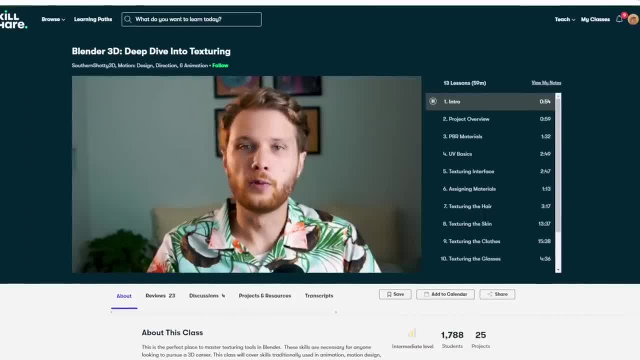 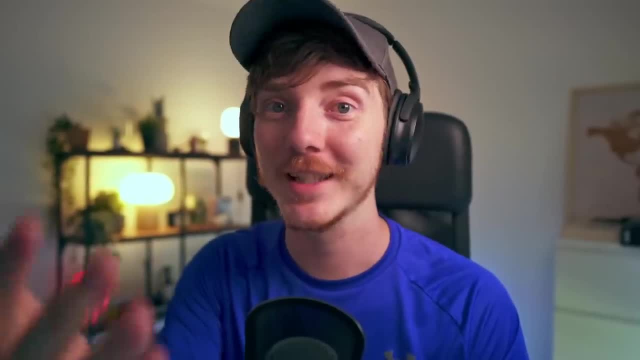 Shoddy's collective classes here. Each of these are under an hour long, extremely easy to follow and will get you super comfortable with Blender. If you're still watching this and aren't convinced, then Skillshare has hooked me up with an amazing offer for you: The first 1000 people to use the 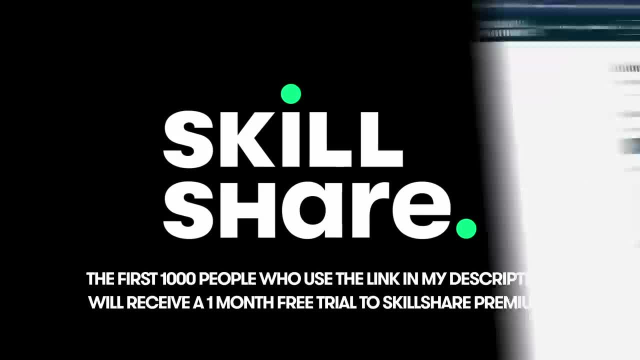 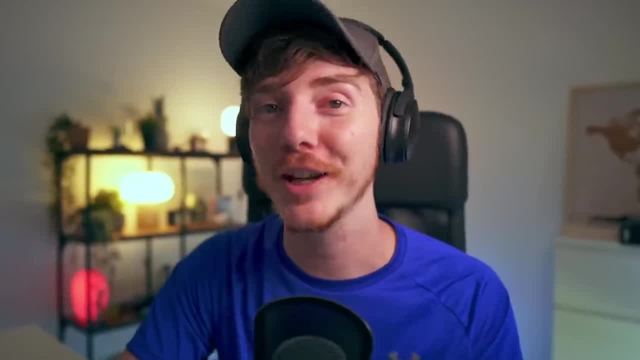 link below will get a full one month free trial of Skillshare. You can binge all of these amazing classes during that time and start getting serious about learning Blender. Grab your free month below and thank you so much to Skillshare for sponsoring this video. So now we know about auto posting and 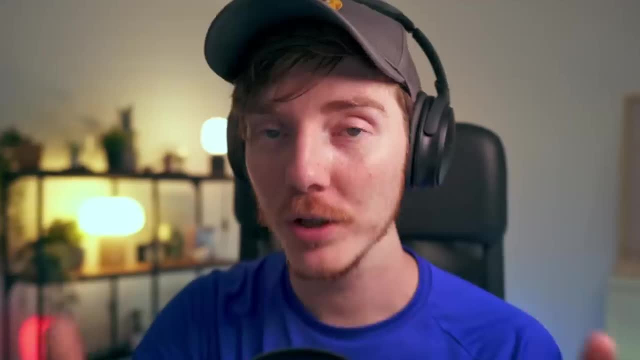 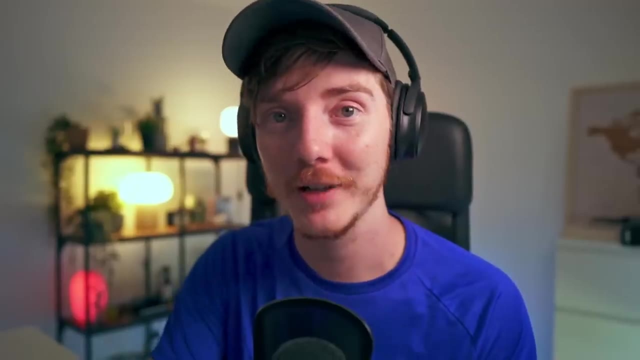 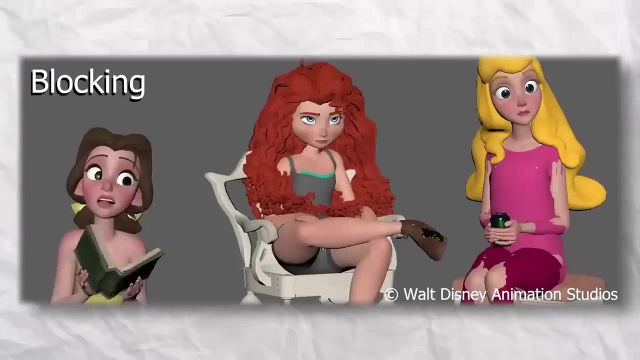 how it can quickly streamline your workflow, but I want to show you the most powerful tool in this software. When you're an animator, some of the most time-consuming activities come in what's known as the polishing stage. This is where your animation is essentially. 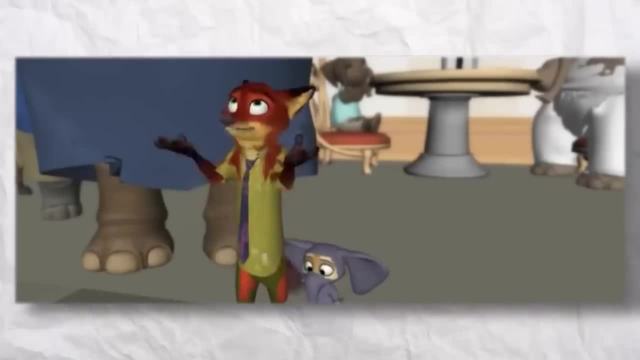 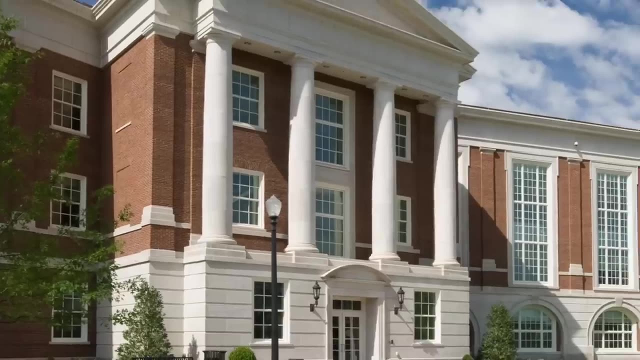 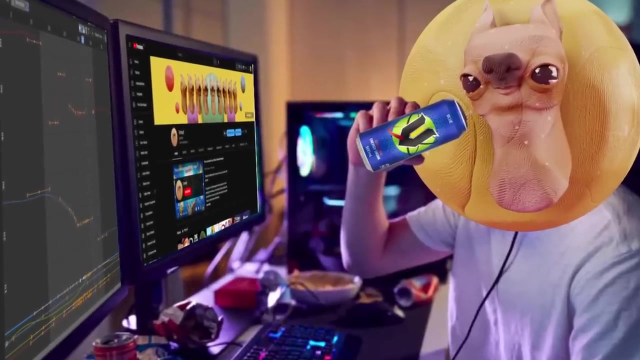 done, but you're adding in small things to elevate it from average quality to insane. I can't tell you enough how painstaking this process can be. I remember in my final trimester of uni I was up all night, drank an unhealthy amount of energy drinks and just trying to cram.